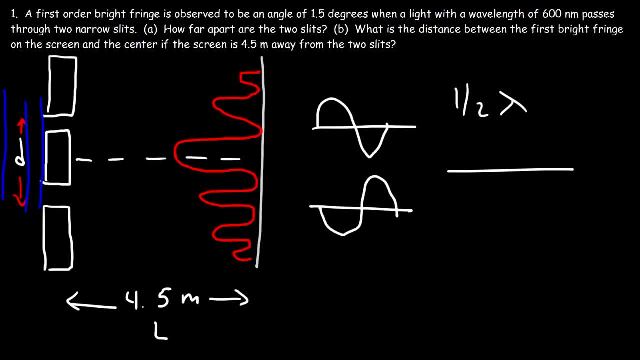 Two waves are out of phase if the wavelengths differ by half, Meaning that they're wavelengths but the relative positions to each other. If their relative positions differ by half a wavelength, то они объ覺ятся по поб Nolan will be out of phase and they will interfere destructively. however, if you 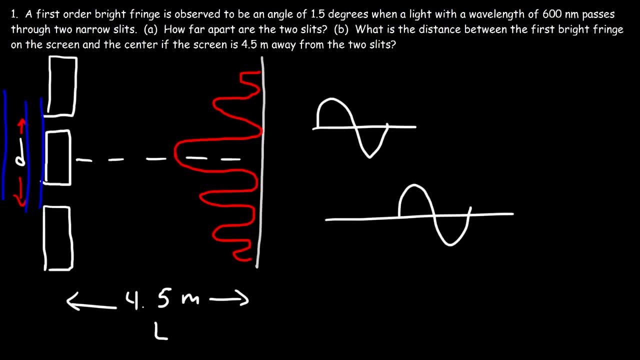 have two waves that are separated by distance of one wavelength, then they will be in phase with each other. now there's two equations that you need to know and we're going to derive them, so let's start with this point. we're going to focus on this point here. so this is one wavelength, two, three, and I didn't 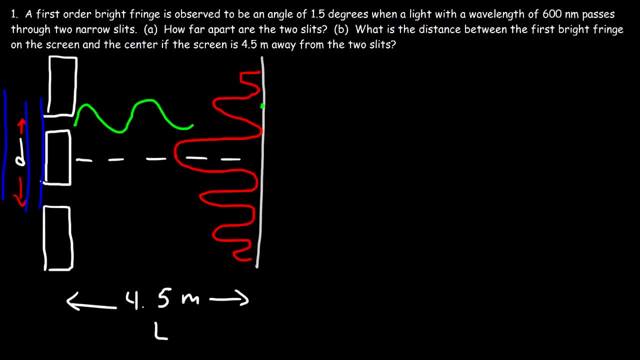 quite make it at three. so let's do that again. let's say this is one, two and then three. and then here it would say: this is one, two, three and then four. now to get to this first fringe, or M is one this way, if requires m. 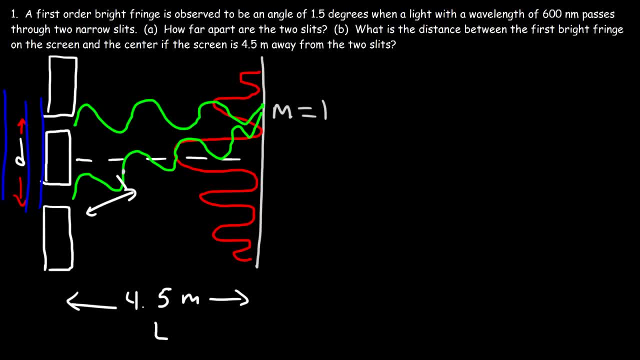 one extra wavelength. And so if we turn this into a right triangle where this is the hypotenuse, this will be the extra wavelength and this distance will be d. So I'm going to redraw that right triangle, So it looks something like this: Here's the hypotenuse, this is 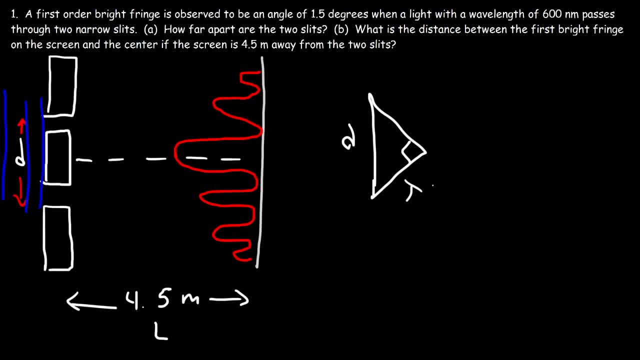 d, and this is lambda, the extra wavelength that was needed for this wave to reach that point. And this is the angle theta which. this will be theta 1.. These two angles are equivalent. This would be theta 2, but we'll talk more about that later. Sine theta is: 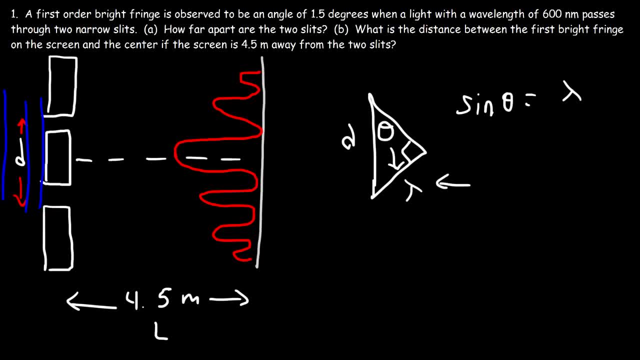 equal to the opposite side. this is opposite to theta divided by the hypotenuse, which is across the box or the right angle. So we have sine theta, which is the opposite side, which is the right angle. So we have sine theta, which is the right angle. So we have sine theta, which is the 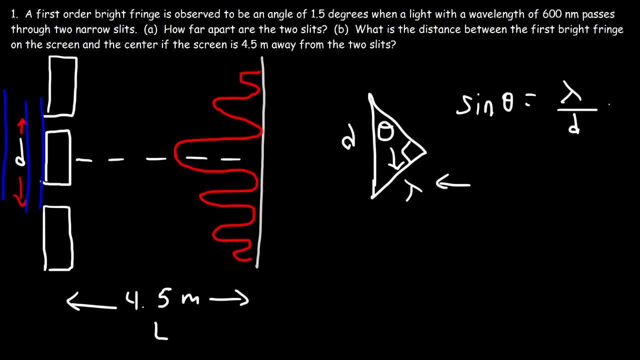 opposite side, which is the opposite side, which is the opposite side. So we have: sine theta equals lambda over d. So if we multiply both sides by d, we get this equation: d sine theta is equal to lambda. Now we need to add m in front of this equation because it 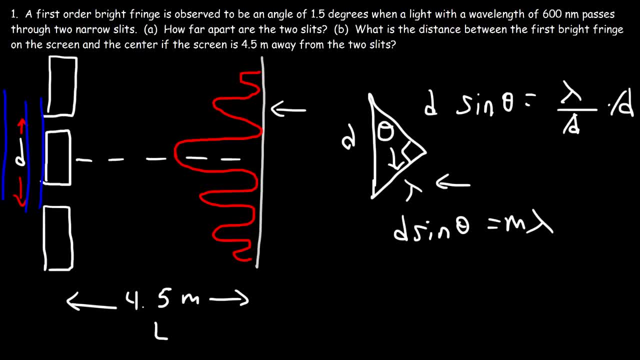 all depends on which fringe we're looking at. So for the first order fringe, m is 1.. For second order, m is 2.. Here, for the one at the center, m is 0. For this one, m is negative 1, and m is negative 2.. So we have: sine theta equals lambda over d. So if we 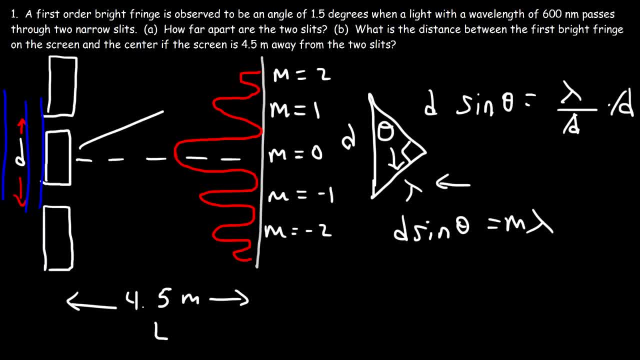 write it negative. we're gonna write d and this is 0.. Where d is negative: 2.. Because at this point these two waves, this one and that one, they will differ by two wavelengths. where m is 2.. Here they will differ by one wavelength. So you need to add m in this equation. 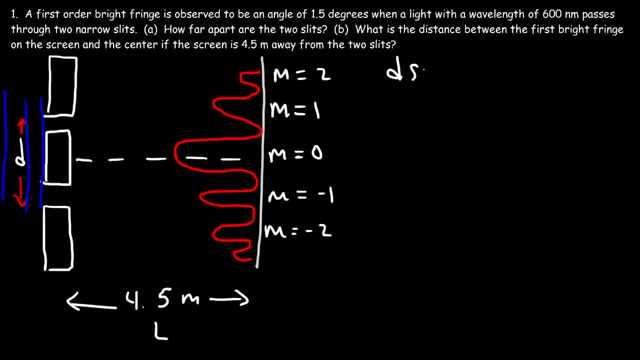 to make it work. So make sure you remember this equation: d sine theta is equal to 1 sine theta, mass m times lambda. So anytime you're given the angle in degrees, you may need to use that formula. Now there's another equation that we need to talk about. So, going from here to here, 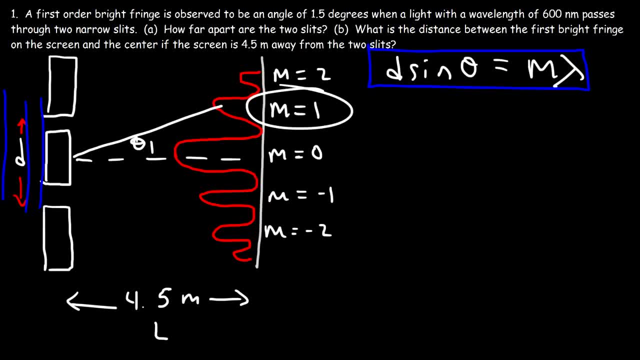 this is going to be theta 1 because it's associated with the first bright fringe And this is L. So we can draw a triangle. Let's say this is theta 1, this is L, And let's call this the distance between the first bright fringe in the center, y1,. 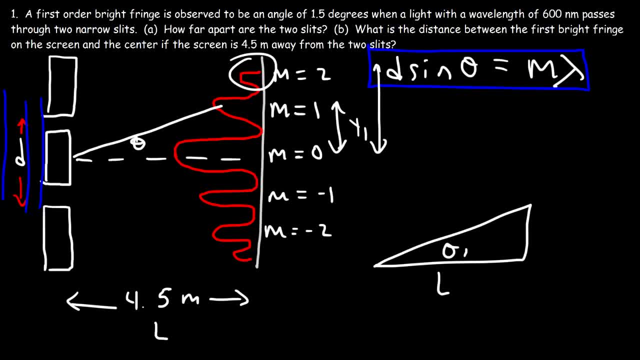 and the distance between the second bright fringe in the center, y2.. So this is y1. in this example, Tangent theta is equal to the opposite side divided by the adjacent side, So it's y1 over L. So that's another formula to know. Now 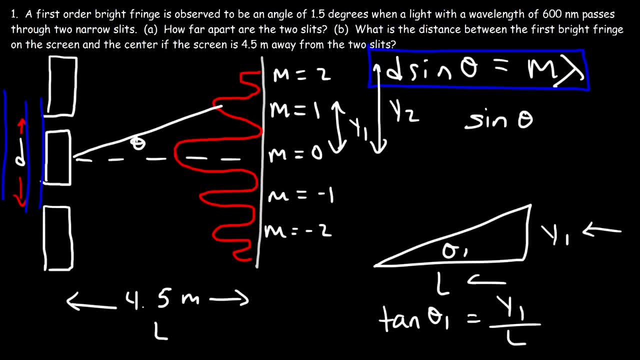 whenever you have an angle, you're going to want to draw a triangle. So in radians, not in degrees, sine theta is approximately equal to theta if theta is very small, And the same is true for tangent theta. It's approximately equal to theta when theta is. 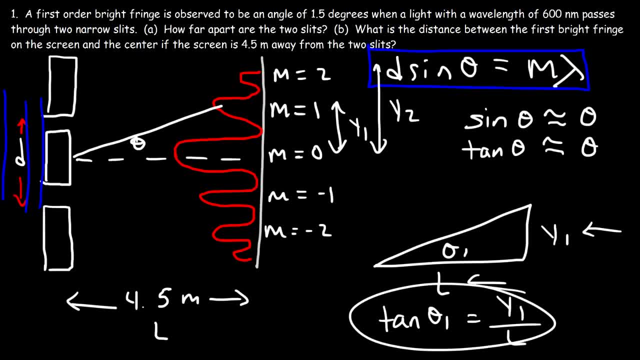 small. So therefore we could say that this formula simplifies to: theta is equal to y divided by L, And this formula simplifies to this d theta is equal to m lambda, And we said that theta is y over L. So then, replacing theta with y over L, we get this. 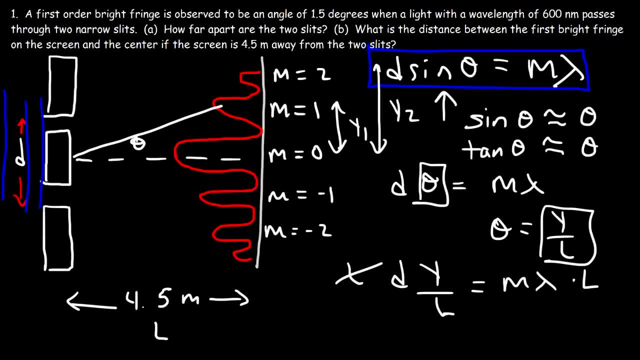 Now I'm going to multiply both sides by L, So this is the form that you want to remember. So y, which I'm going to write y sub m, because it's dependent on this number, times d, the separation distance between the two slits is equal to L m lambda. So this is the second formula that you want to write down. 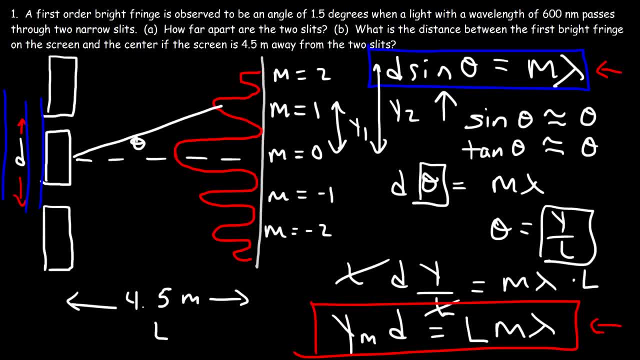 Make sure you know these two, because these are the two equations we're going to be using. Now let's go ahead and finish this problem. So, part a: how far apart are the two slits? Let's make a list of what we know. 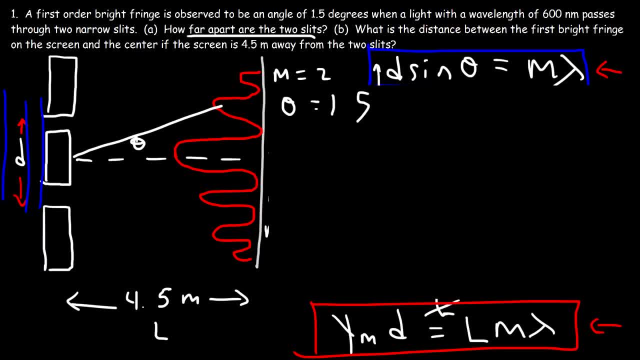 So we know that theta is 1.5 degrees And we also know that lambda is 600 nanometers. That's the wavelength. Our goal is to calculate the distance between the two slits And we have a first order: bright fringe, which means that this is first order. m is 1.. 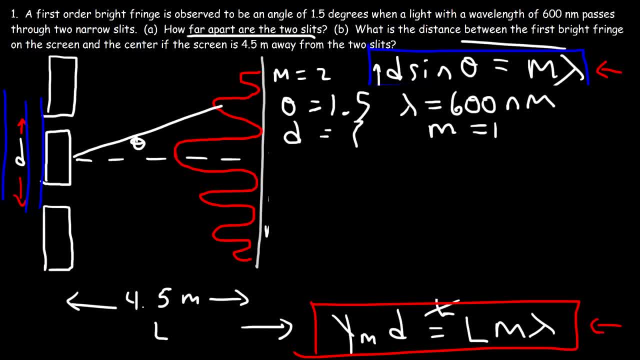 So for this first part, we don't need this equation, We only need this one, So let's go ahead and use it. So we need to calculate: D, Theta is 1.5 degrees, M is 1. And lambda is 600 nanometers, or 600 times 10 to the minus 9 meters. 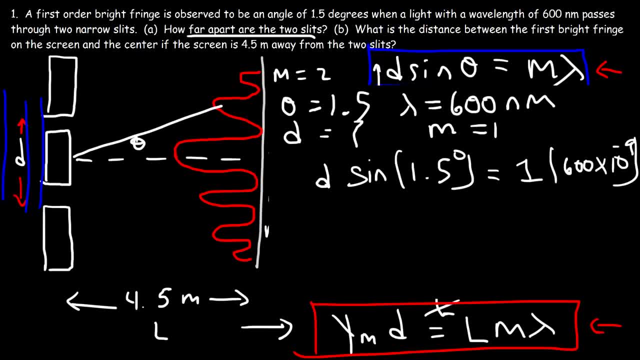 So 600 times 10 to the minus 9, divided by sine of 1.5. That's equal to 2.29 times 10 to the minus 5 meters, And if you divide it by 10 to the minus 3, this is going to be 0.0229 millimeters. 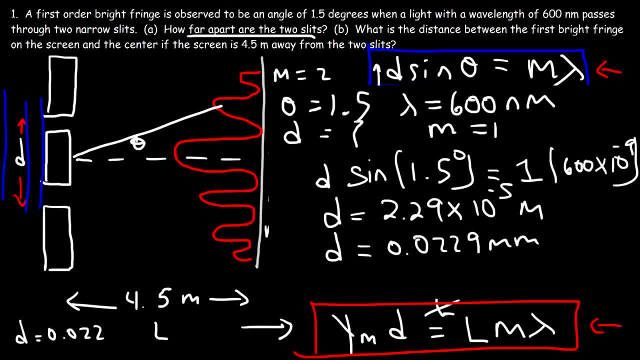 So I'm just going to write that here. Now let's move on to part B. What is the distance between the first bright fringe on the screen and the center if the screen is 4.5 meters away from the slit? So this is the screen. 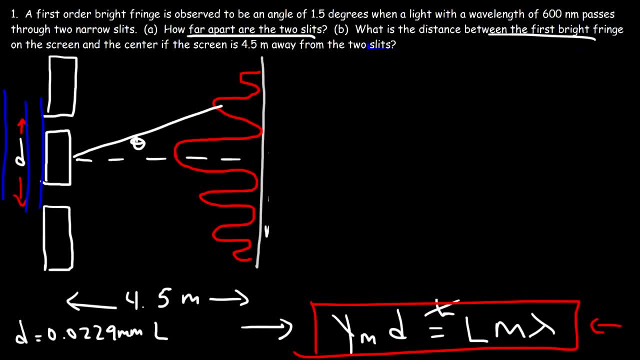 So here is the first bright fringe. That's where M is equal to 1.. So we need to calculate this distance between the first bright fringe and the center. So basically Y1.. So let's use this formula. So in this case M is 1.. 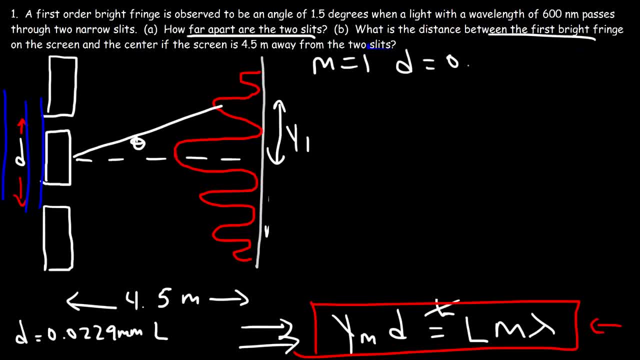 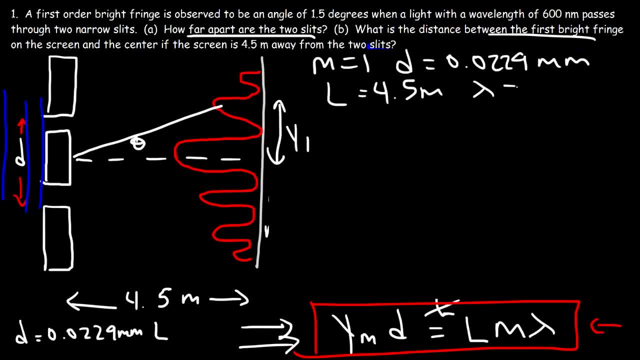 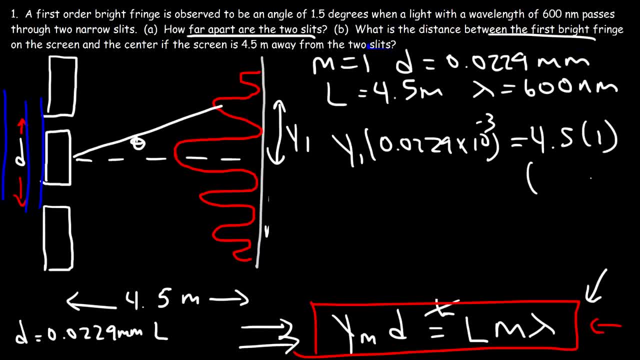 That's equal to L times M times lambda, which is 600 times 10 to the minus 9.. L. So let's multiply 600 times 10 to the minus 9 by 4.5.. And then divide that result by 0.0229 times 10 to the minus 3.. 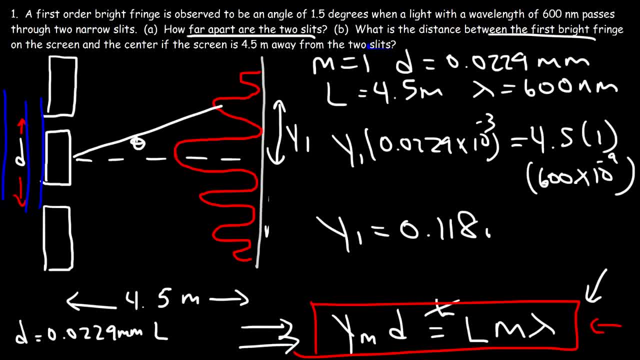 And so Y1 is 0.118 meters, or you could say 11.8 centimeters. So that's how far the first bright fringe is from the center. Go ahead and try this problem. Light with a wavelength of 0.0229. 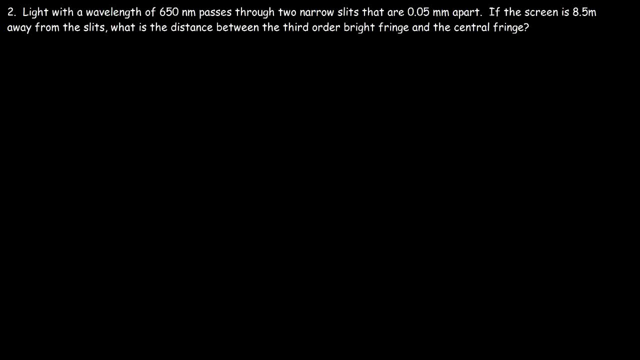 So let's say that the wavelength of 650 nanometers passes through two narrow slits that are 0.05 millimeters apart. If the screen is 8.5 meters away from the slits, what is the distance between a third order bright fringe and a central fringe? 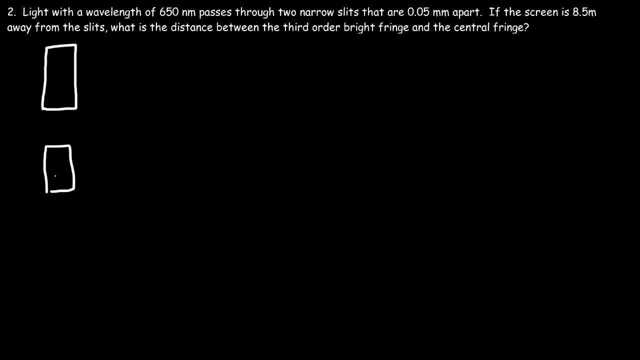 So let's start with a picture. So let's say that this is the screen And it's 8.5 meters away From the slits, And so this is going to be the central bright fringe. There's the first fringe, second and then the third. 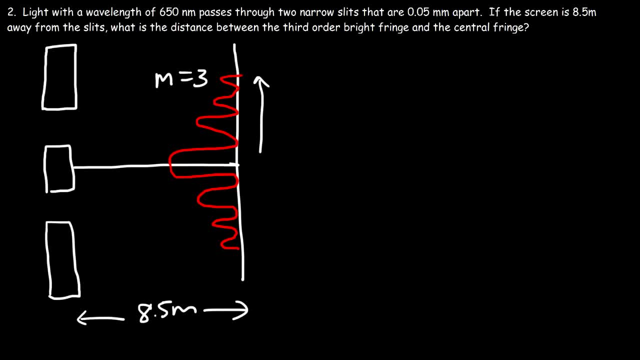 So here M is equal to 3. And so we want to find out how far the third fringe is from the central fringe, And we're given D the distance between the two slits. So D is 0.05 millimeters. 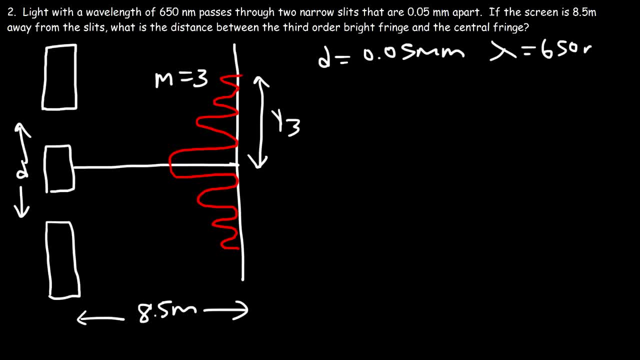 And then lambda is 650 nanometers, L is 8.5 meters And we're dealing with the third order, bright fringe. so M is 3.. So let's use this formula again: YM times D is equal to LM Times- lambda. 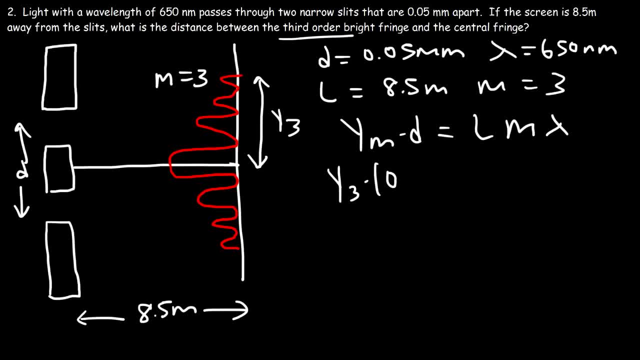 So we're looking for Y3.. D is 0.05 millimeters, Or 0.05 times 10 to the minus 3.. L is 8.5.. And then times M, which is 3.. Times lambda, which is 650 times 10 to the negative 9.. 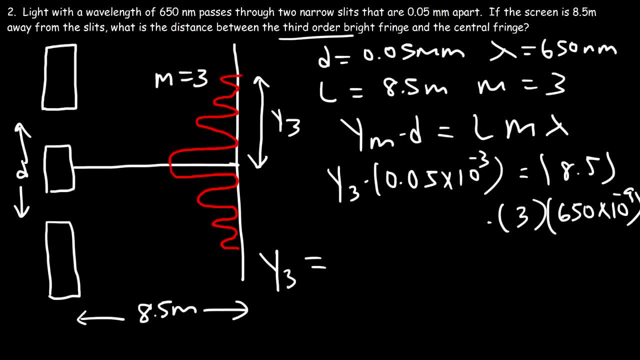 So what we need to do is take 8.5.. Multiply it by 3. And multiply that by 650.. Times 10 to the minus 9.. And then take that result, Divide it by 0.05 times 10 to the negative 3.. 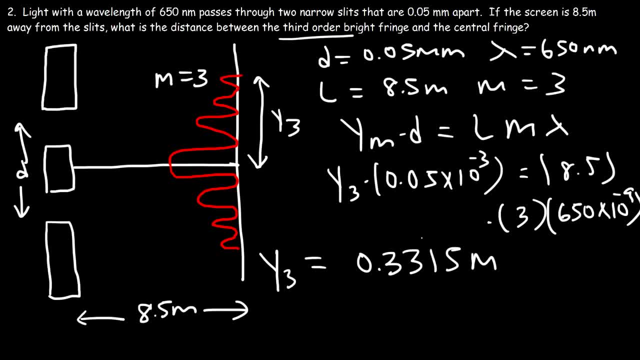 And so Y3 is going to be 0.3315 meters away from the central fringe. So that's the answer. Or if you want it in centimeters, you could say it's 33.15 centimeters. Just multiply this by 100. 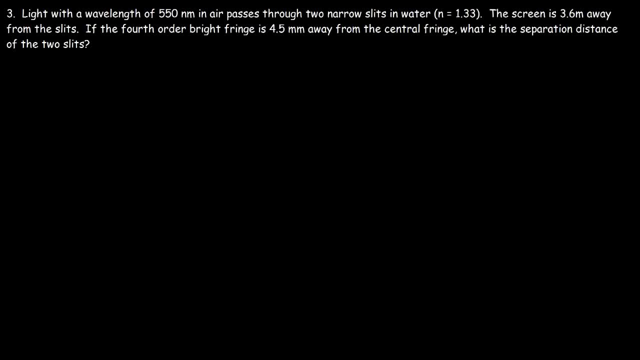 And so that's it for this problem. Number 3. Light with a wavelength of 550 nanometers. Light with a wavelength of 550 nanometers In air Passes through two narrow slits in water, And we're given the index of refraction of water. 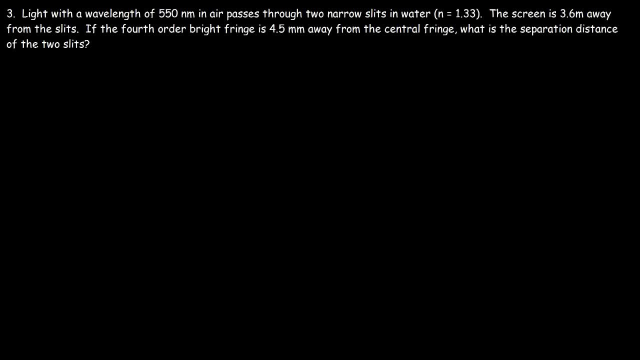 The screen is 3.6 meters away from the slits. If the fourth order bright fringe is 4.5 millimeters away from the central fringe, What is the separation distance of the two slits? Go ahead and pause the video. 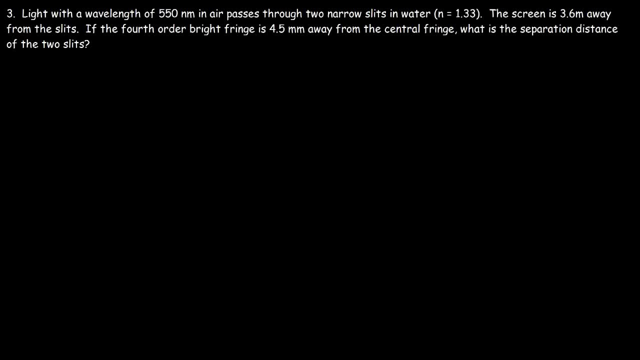 Feel free to try this problem if you want to. So we're given the wavelength in air, That's 550 nanometers. That's 350 nanometers. We have the index of refraction, We have the length, which is 3.6 meters away from the two slits. 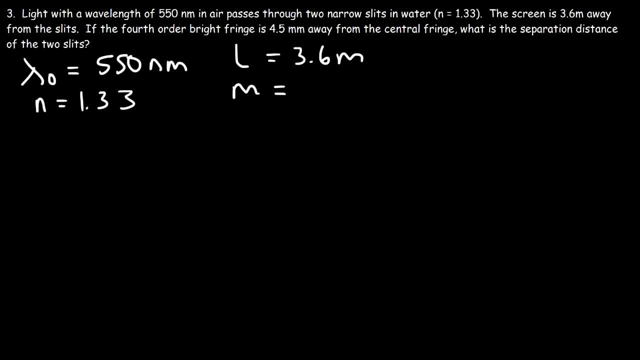 And we also have m. We're dealing with a fourth order, bright fringe, So m is 4.. And the distance between the fourth fringe and the central fringe is 4.5 millimeters. So that's Ym, which is Y4.. 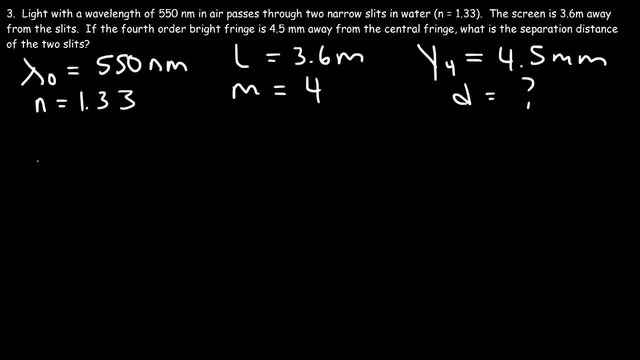 So we need to calculate D, So we need to use this formula: Ym times D is equal to Lm times lambda. So how do we incorporate N in this problem? You need to know that, as light moves from a material with a low index of refraction, 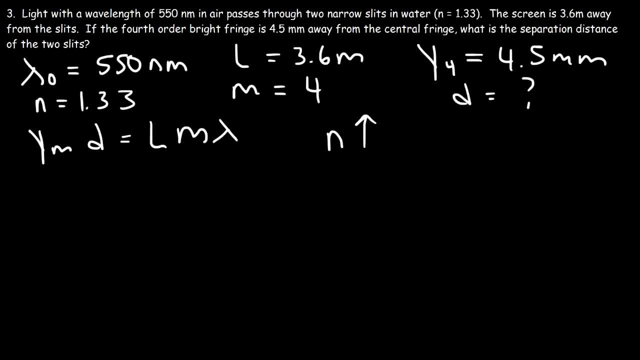 to a material with a higher index of refraction, the wavelength of the light decreases. So we need to calculate the new wavelength of light using this formula. So it's going to be 550 nanometers divided by 1.33.. And so the wavelength of light in water is 413.5 nanometers. 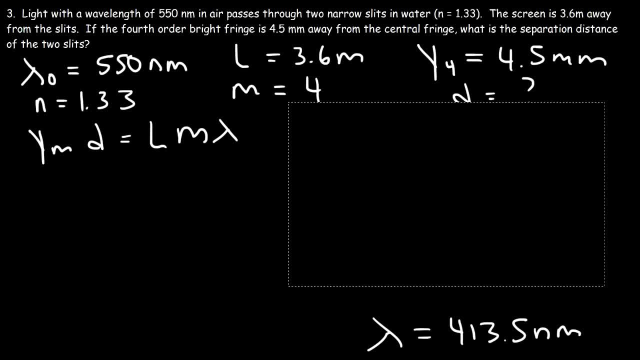 So now we can finish the problem. So Ym or Y4, is 4.5 millimeters, or 4.5 times 10 to the minus 3 meters. Our goal is to calculate D, the separation distance of the two slits. 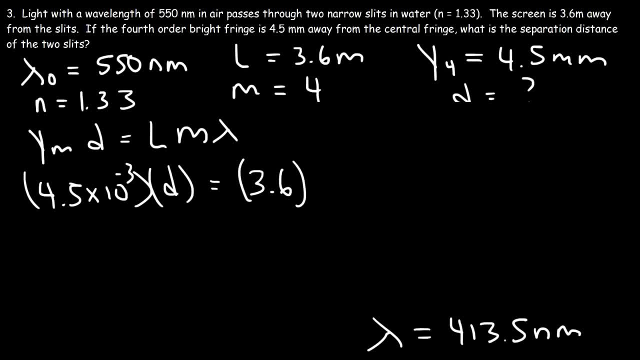 L, the distance between the screen and the two slits, that's 3.6 meters, M is 4, and lambda is this value 413.5.. Times 10 to the minus 9 meters, So 3.6 times 4 times 413.5. times 10 to the minus 9.. 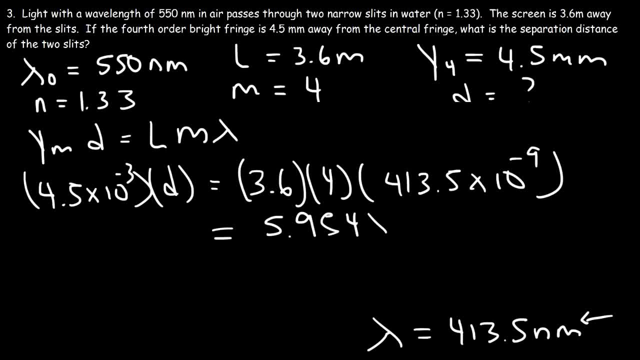 All of that is equal to 5.954 times 10 to the minus 6.. And so we need to take that answer and divide it by 4.5 times 10 to the minus 3.. And so the separation distance between the two slits is 1.32 times 10 to the minus 3 meters. 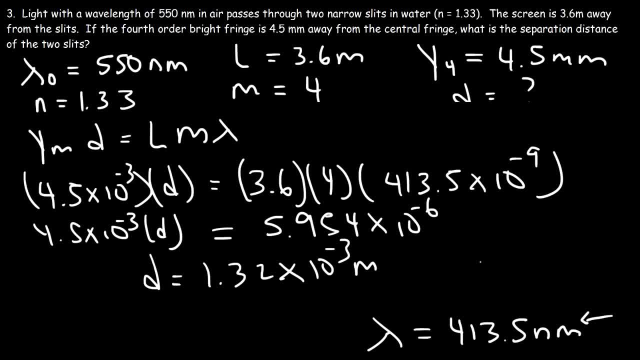 And 10 to the minus 3 is basically a millimeter. So this is 1.32 millimeters, And so that's the separation distance of the two slits. So remember, for these types of problems there's only two formulas you need.